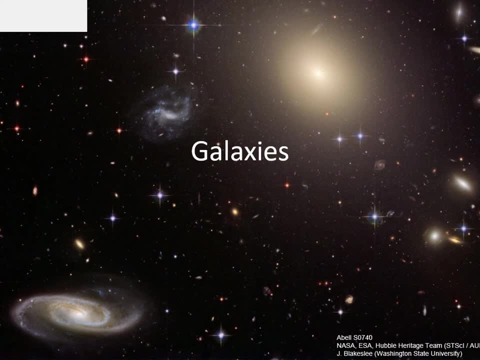 that shape galaxies, even if we don't have time for a detailed discussion of all of the structures we find in them. Just as stars are the most obvious building blocks making up a galaxy, galaxies are the most obvious building blocks making up the larger universe. As a result, we're not just 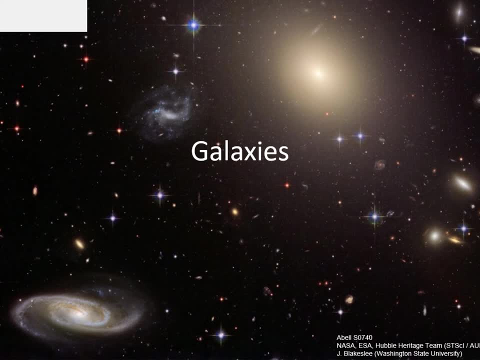 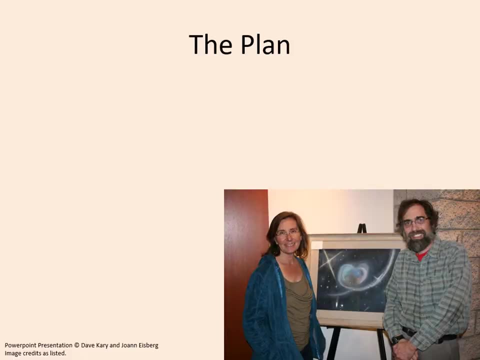 interested in galaxies themselves, but also in what they can tell us about the distribution of mass and energy in the universe as a whole. We'll start looking at galaxies by seeing the major types of galaxies we can observe around us, and we'll notice what makes them different from each other. 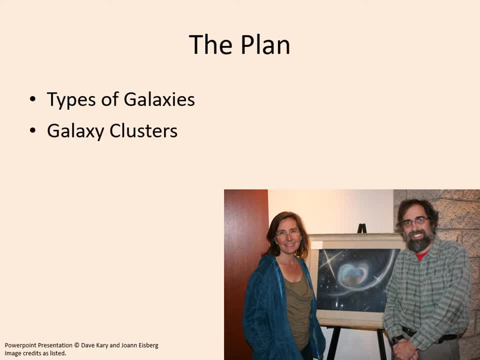 Then we'll see that, just like with stars, galaxies often come in groups or clusters. Next we'll see how we measure distances in astronomy. Some of this will be reviewed from earlier chapters, but we'll add several more steps as we compare the different techniques. 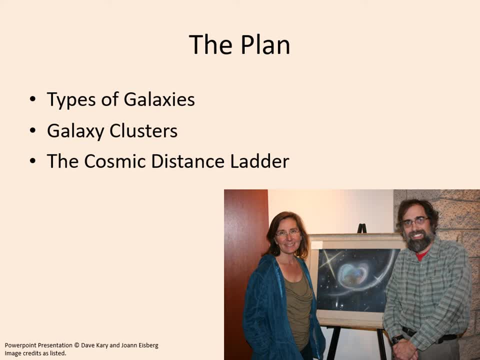 used to measure distances to stars and galaxies. Once we know the distances to galaxies, we can look at one of the most important discoveries in astronomy in the last century – the expansion of the universe. There are many implications of this expansion, some of which will wait until a later chapter. 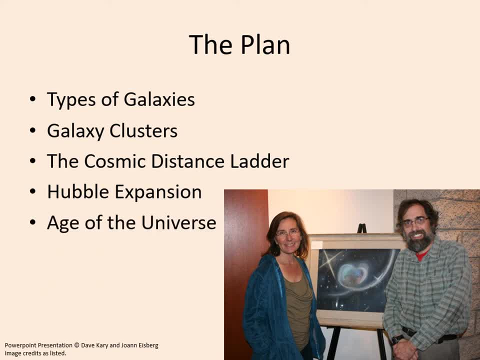 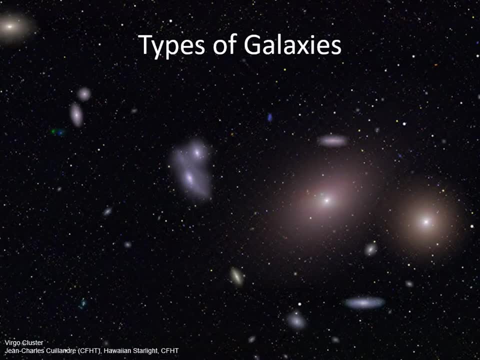 however, one key result we can discuss now is the age of the universe, which we can calculate directly from the expansion. Galaxies are much more complex than stars and, over the years, astronomers have come up with several different ways of classifying galaxies. However, we're going to use the 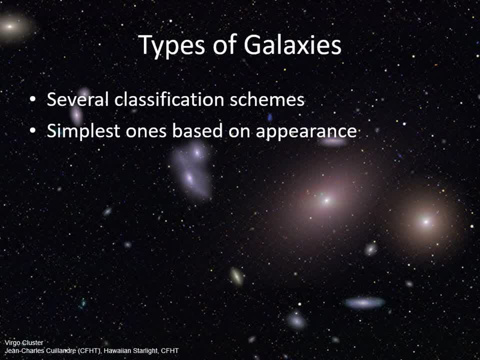 simplest and most common classification system- wwwciallyoutubecom, http//wwwyoutubecom, http//wwwyoutubecom, http//wwwyoutubecom, http//wwwyoutubecom, http//wwwyoutubecom, scheme which divides galaxies up into just a few broad categories based on their appearance. 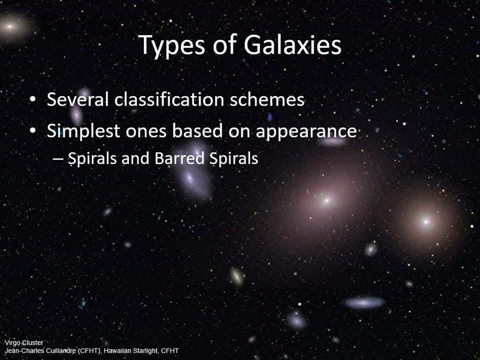 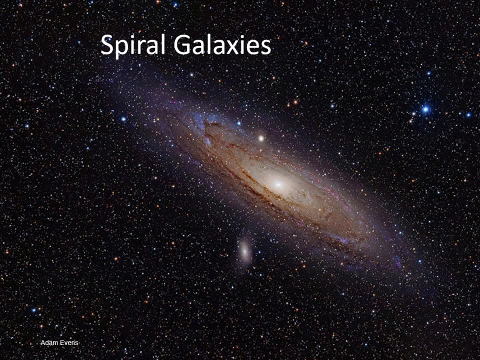 These categories are spirals and barred spirals, ellipticals, lenticulars and irregular galaxies. We'll look into each of these types in the next few slides. One of the most common types of galaxies around us is spiral galaxies. The structure we've already seen for the Milky Way applies to spiral galaxies in general. 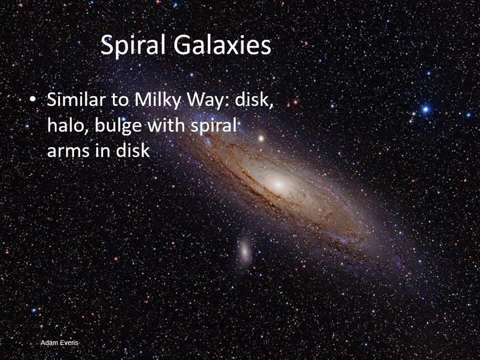 There is a bulge, halo and disk with active star formation along the spiral arms in the disk. The active star formation means that much of the light from these galaxies comes from the hot, high-mass main-sequence stars, making the galaxy relatively blue, especially in the disk. 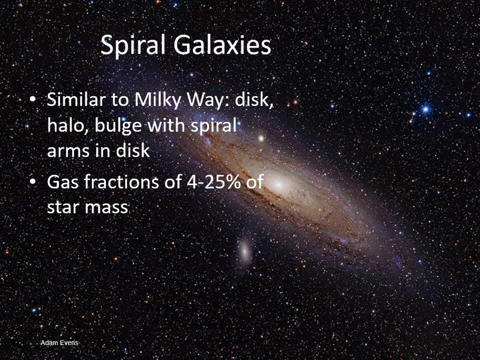 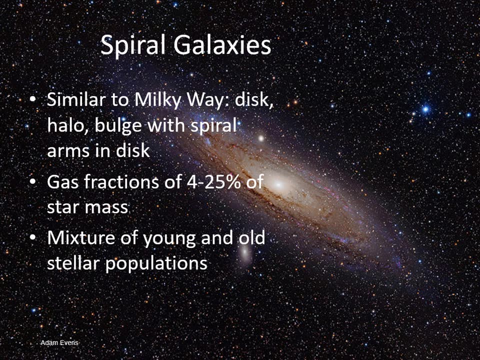 Typically between 4 and 25 degrees Celsius. 25% of the visible mass of a spiral galaxy is in the form of gas. It's this gas that fuels the active star formation. Since stars are currently forming, there's a mixture of both old and young stars, especially. 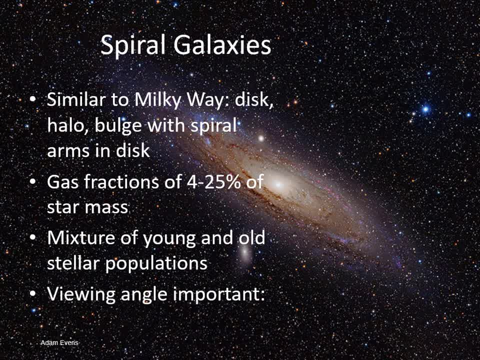 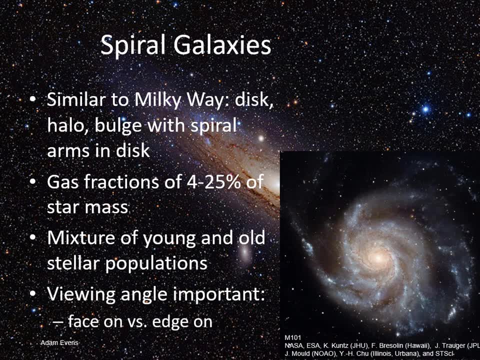 in the disk. The appearance of a spiral galaxy will depend on the viewing angle we have for it. With a face-on spiral, we see the pattern of spiral arms surrounding the central bulge. If the galaxy is edge-on, it's a spiral. 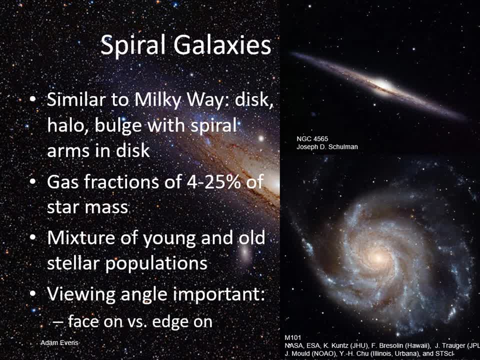 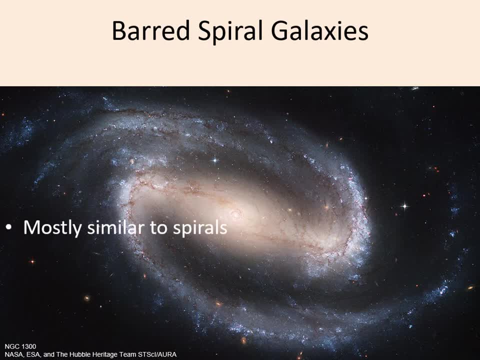 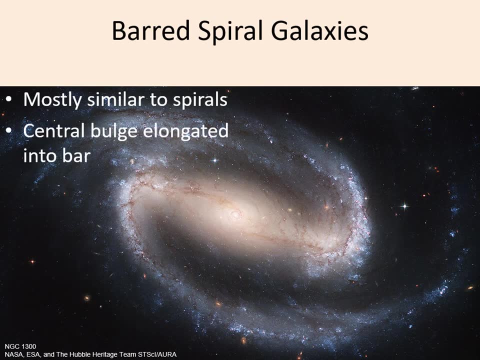 The dust in the disk cuts across the central bulge and we may see some of the globular clusters surrounding the bulge. Barred spirals are similar to spiral galaxies. The one thing that distinguishes them is that the central bulge is stretched out into a 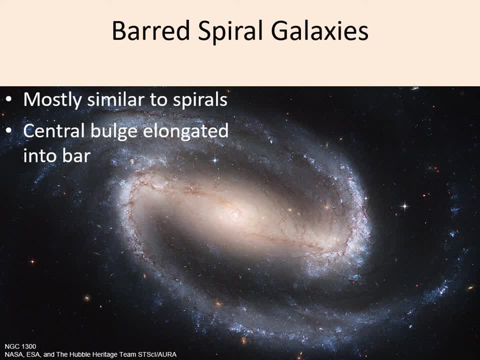 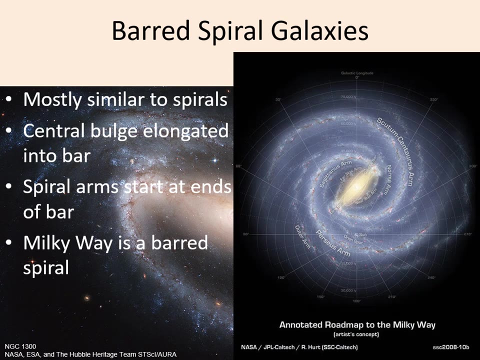 bar shape. Since this bar generates the disturbance that causes a spiral density wave in the galaxy's gas, the spiral arms typically start from the ends of the bar. The spiral arms typically start from the ends of the bar. As we've already seen, the Milky Way is an example of a barred spiral galaxy. 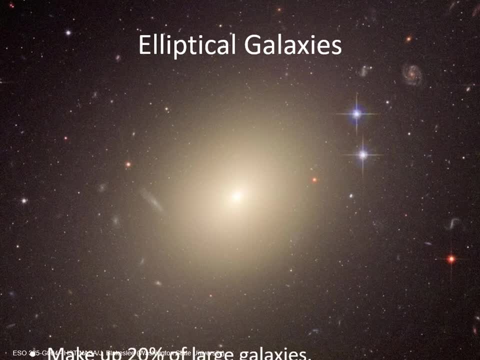 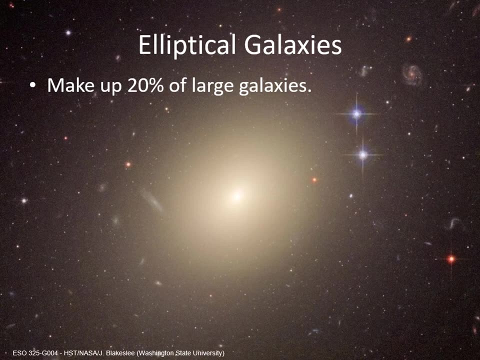 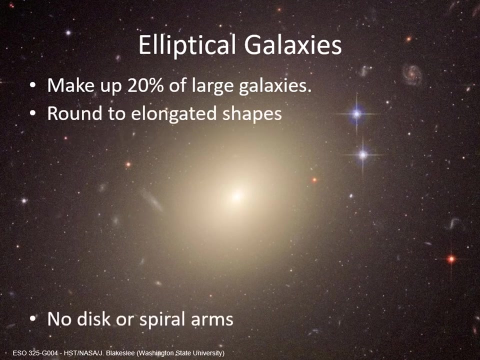 The next most common type of galaxy is ellipticals. These galaxies make up roughly 20% of all the large galaxies we see, and they're an even larger fraction of the small galaxies. When we see ellipticals, they can be either circular or elongated in shape, but they show. 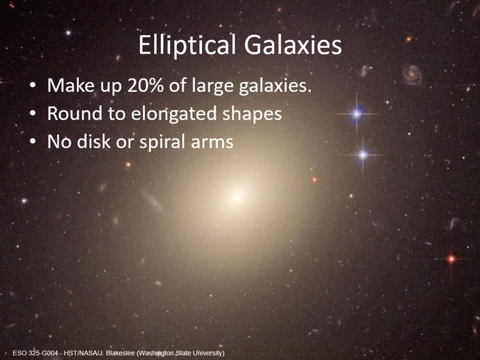 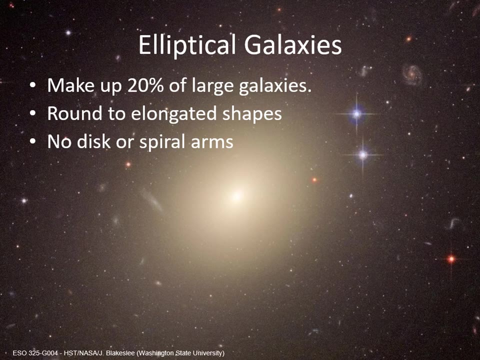 no sign of a disk or spiral arms. When we see a round-shaped elliptical, they're a spiral. When we see a round elliptical galaxy, it could be spherical or elongated, with the long axis pointing towards the star. With no disk, there isn't any easy way to tell what the orientation of the system is. 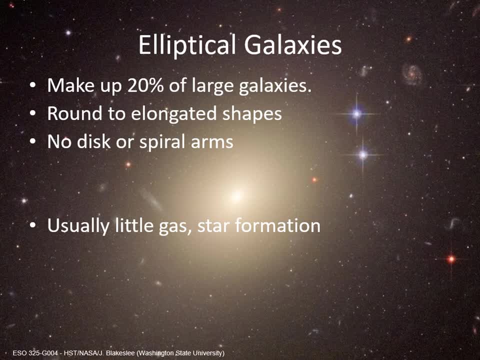 Elliptical galaxies usually have little or no gas, so there usually isn't any active star formation in these galaxies. As a result, these stars are mostly Population II and VERY old population stars. This is what these stars look like. This is mostly Population I and II. The никeness of the stars is what these stars are called in stars. Not all stars are likely to remain than the D of the star India". Alibaba said. The nutzen of total stars? By and large, neither any star forms found in areas of life or limits estavaissimum. 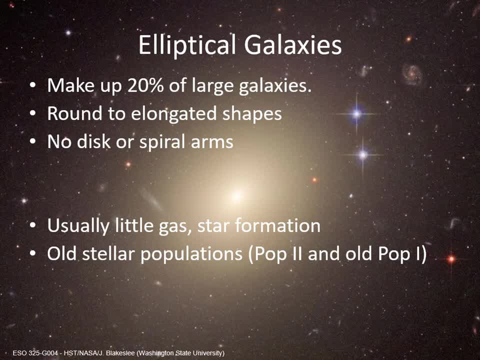 monitor over two Craven's system, the Sun'sテ, Butte's lucky damsel, one stars and, just like globular clusters, the light is usually dominated by red giant stars. Elliptical galaxies include both the very largest and the very smallest galaxies. we 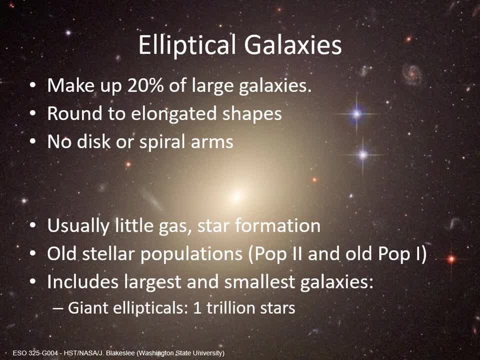 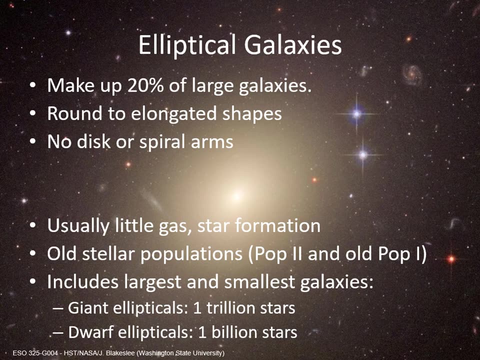 see. The largest giant ellipticals can have a trillion stars in them, several times the number in the Milky Way. On the other hand, the smallest dwarf elliptical galaxies can have less than a billion stars in them, less than 1% of the size of our galaxy. 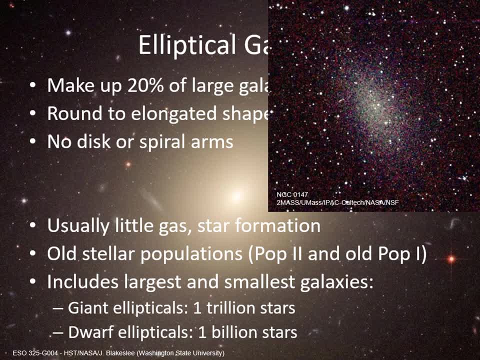 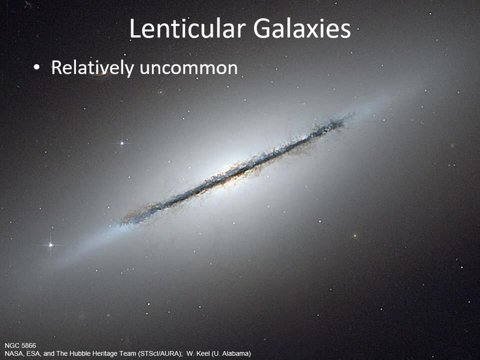 Small, faint galaxies like this are often spread out enough that they're barely visible against the background, so we usually only see the very closest of these dwarf galaxies. Lenticular galaxies are much rarer than spirals or ellipticals. At first glance they often look like spiral galaxies. 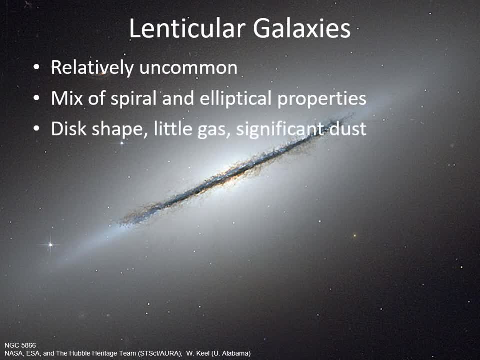 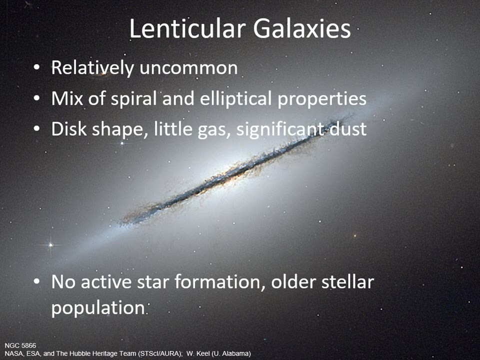 However, while they have a disk, there is very little gas in that disk, though there may be a larger-than-average fraction of dust. The lack of gas means that there is very little star formation and the population of stars is typically much older than in the disks of spiral galaxies. 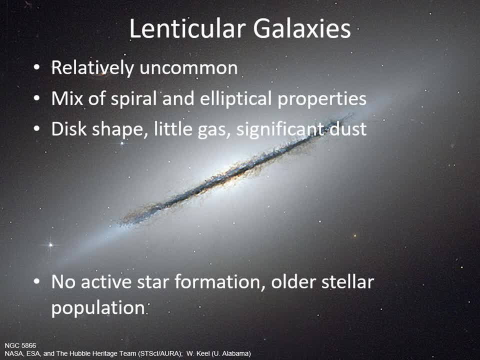 This suggests that early in the galaxy's history, most of the gas was converted into stars, Just a small amount later ejected as stars die. Also, since there's very little star formation, there are no spiral arms. However, lenticulars do have a central bolt. 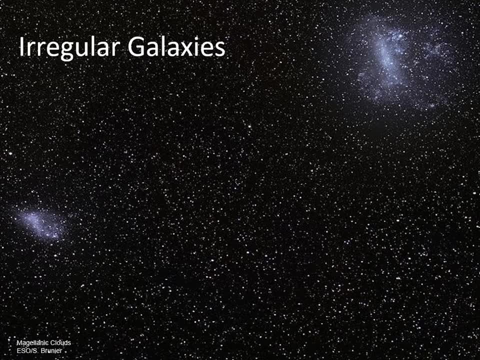 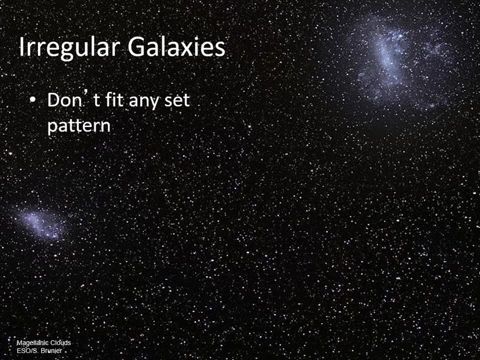 The remaining class of galaxies is a catch-all category known as irregular galaxies. These don't follow any of the standard classes described above and many don't have any clearly defined shape. At the small end of this category, there are no spiral arms. 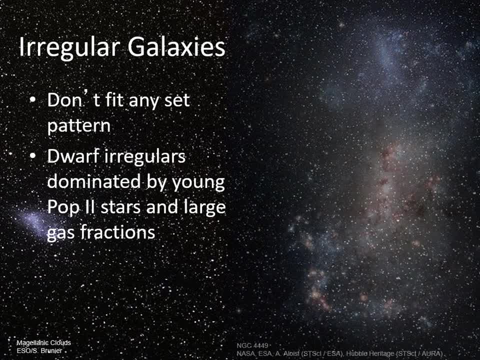 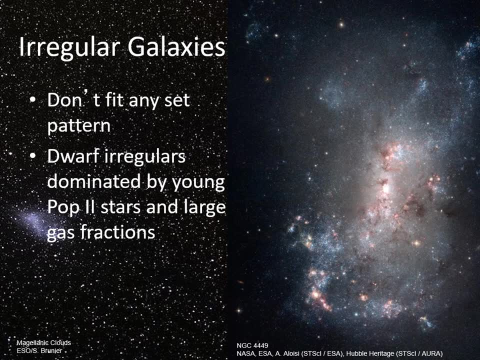 There are no spiral arms. The dwarf irregulars like the one shown here often have 25% or more of their mass in the form of gas. This high gas fraction means that there is plenty of active star formation and the stellar population is dominated by young population 2 stars, in other words, young stars with 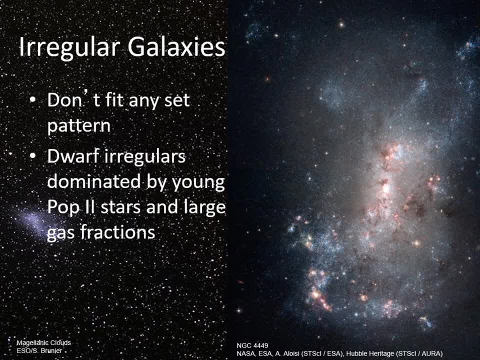 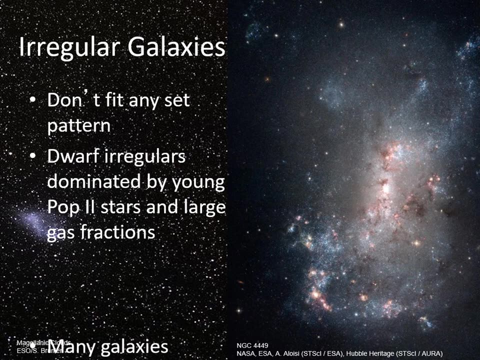 very few metals in them. This suggests that the star-gas-star cycle hasn't been converting gas into stars very efficiently over time, and hence the gas isn't contaminated with metals the way it is in spirals. Many irregular galaxies also show signs of being distorted by collisions. 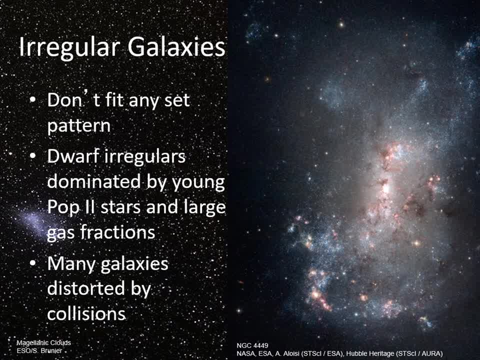 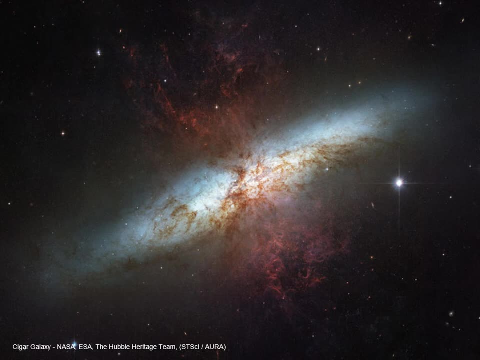 As we'll see later, galaxy collisions are fairly common and, since they can take hundreds of millions of years, we only see a brief snapshot as the galaxies respond to the interaction. For example, This galaxy has suffered a recent collision that caused clumps of rapid star formation. 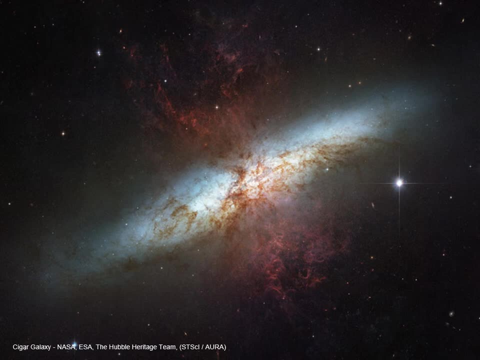 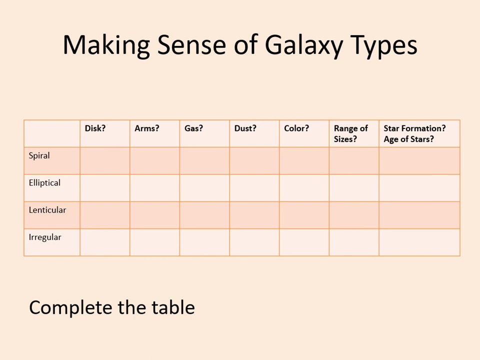 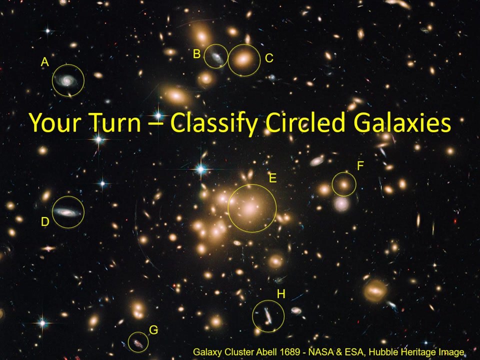 and large jets of gas extending out into the galaxy's halo. Now review the material we've covered to fill in this table on the different types of galaxies. Now it's your turn to classify the circled galaxies in this Hubble Space Telescope image of galaxy cluster Abel 1689. 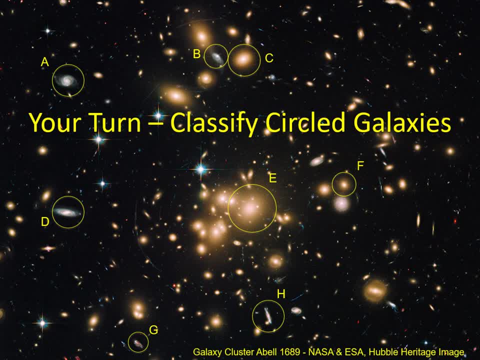 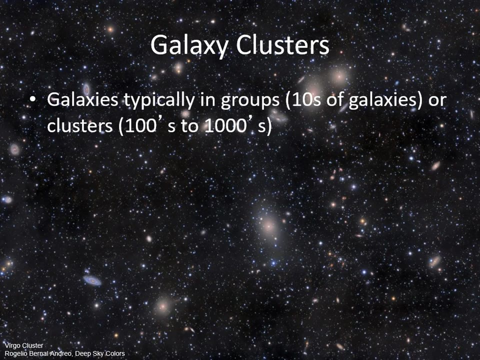 Some are ambiguous. You'll need to explain your choices. Remember that color and shape are both useful criteria. Also, pick out the central dominant galaxy in this cluster. Galaxies are social creatures. They typically come in small groups with a few tens of members located over a few. 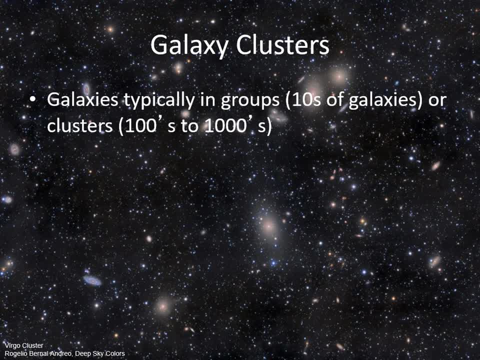 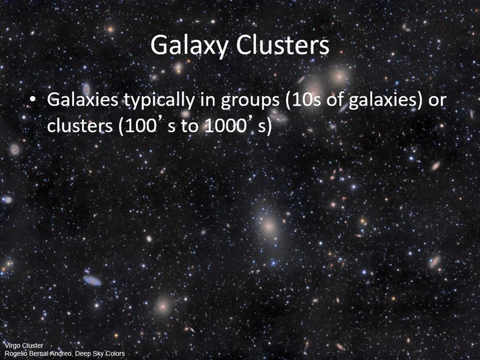 million light years, or in larger clusters with hundreds to thousands of galaxies stretched over tens of millions of light years. When a galaxy is in a cluster, it takes billions of years to move through that cluster, pulled by the gravity of the other galaxies. 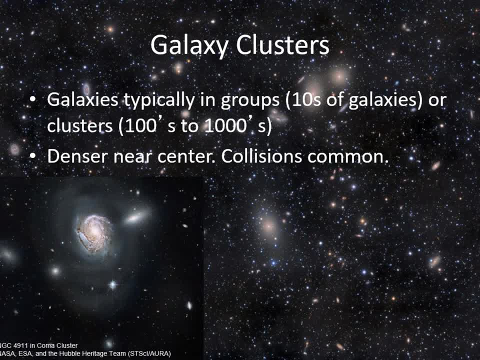 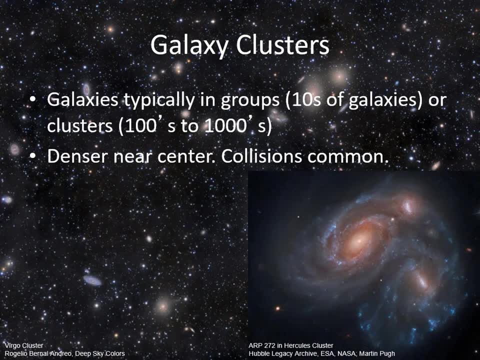 The densest part of a galaxy cluster is near the center. Here the galaxies crowd together and they often collide with each other, as with these galaxies in the Hercules cluster. Often at the center of a cluster there are one or two giant elliptical galaxies. 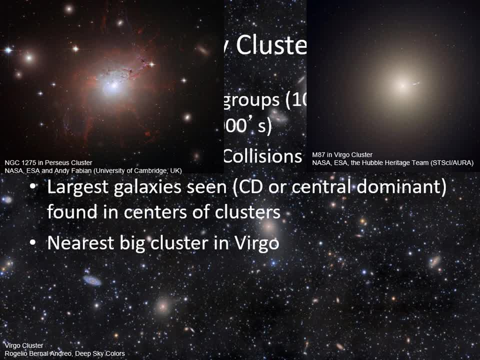 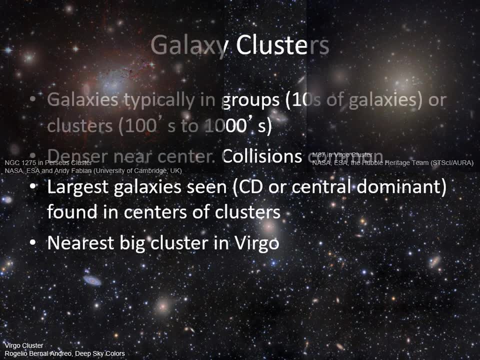 These are referred to as central, dominant or CD galaxies. These are called central, dominant or CD galaxies. These are called central, dominant or CD galaxies And they're probably the result of the merger of many ordinary-sized galaxies. Our Milky Way is in a small group of galaxies near the edge of the much larger Virgo cluster. 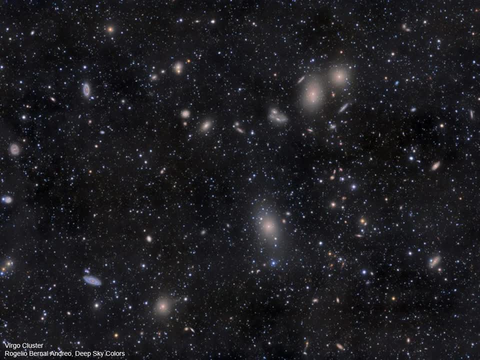 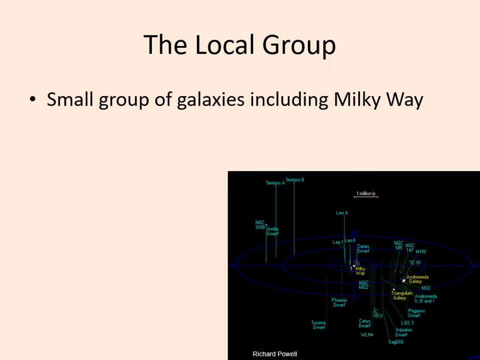 This picture shows the center of the Virgo cluster, about 60 million light years away. As we just said, the Milky Way is in a small group of galaxies that we've creatively named the Local Group. The Local Group has roughly 40 members. 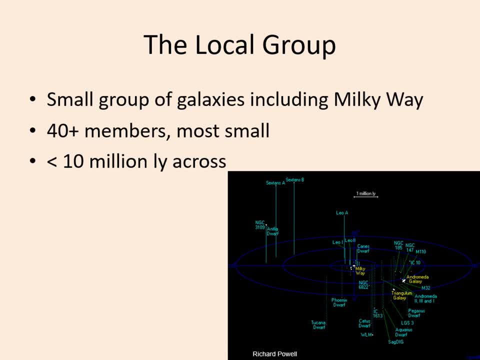 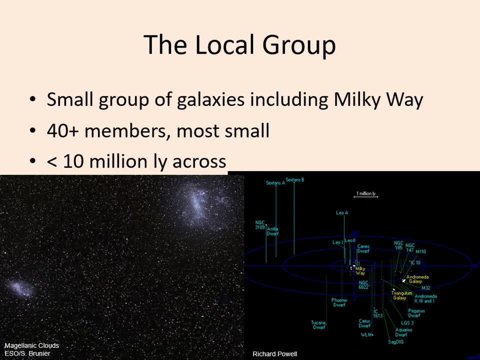 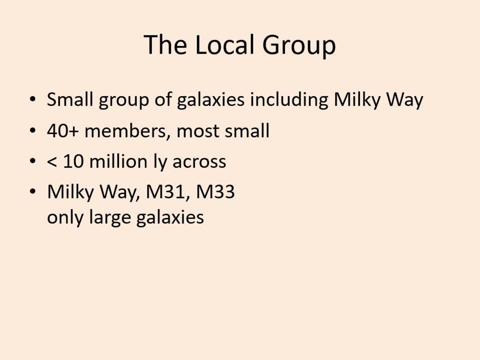 And they range in less than 10 million light years across. Most galaxies in this group are small satellites of the larger galaxies. The Large and Small Magellanic Clouds are two of these. They orbit the Milky Way. Only three could be considered large galaxies. 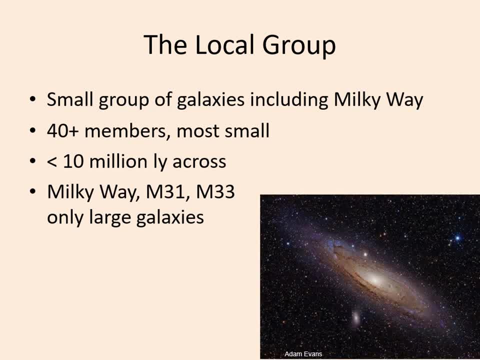 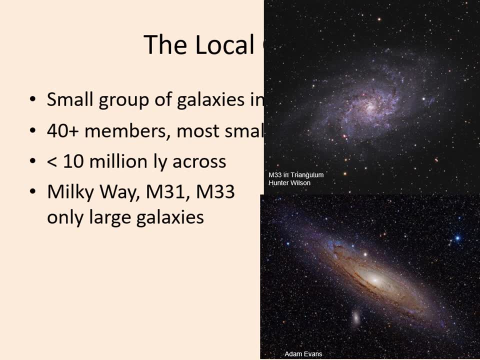 The Milky Way, M31,, which is also known as the Great Galaxy in Andromeda, and M33,, a slightly smaller galaxy in Triangulum. These galaxies are called the Large Galaxy, And the Large and Small Magellanic Clouds are two of these. 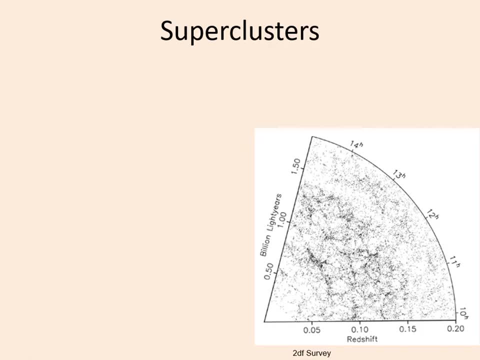 galaxies is bigger than all of the smaller ones combined. When we look at the universe on still larger scales, we see that clusters of galaxies combine into much bigger structures called superclusters. Superclusters are enormous. They can have hundreds of thousands of galaxies in a region up to a billion light years across. In this map of a region of the local universe: 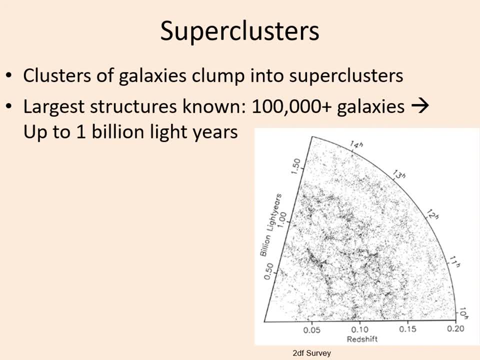 the Milky Way is the point on the far left side, and each yellow dot represents a galaxy. At these distances we're only plotting the biggest and brightest galaxies. so even here it's just a small sampling of all the galaxies in the region. Notice the bright yellow clumps. 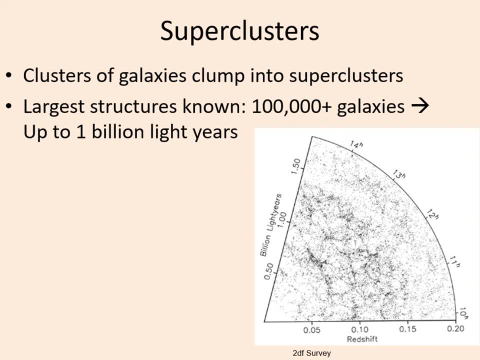 and filaments of galaxies stretched across hundreds of millions of light years. In between these filaments there are voids with very few galaxies. The shape of these clumps and voids gives us clues about the formation and evolution of the universe as a whole. Subtitles by the Amaraorg community.